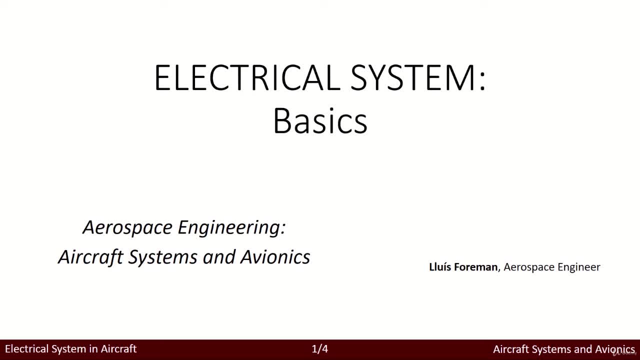 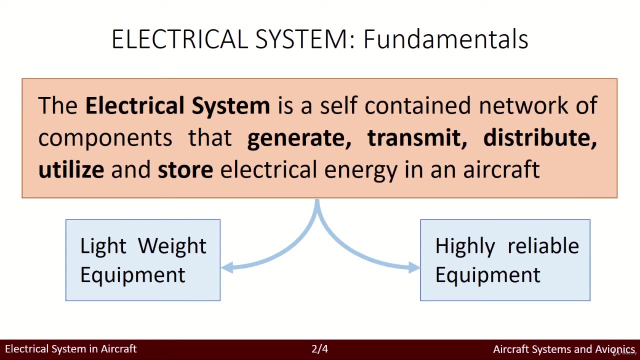 Hey guys, and welcome to this new section in this course in aircraft systems and avionics. Today we will start by introducing and studying the basics of the electrical system. Right, so the definition of the electrical system is a self-contained network of components that generate, transmit, distribute, utilize and store electrical energy in an aircraft. 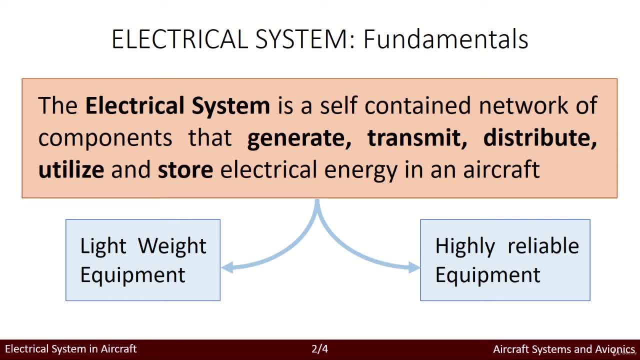 Now, electrical design in aircraft is influenced always by two basic requirements: The equipment must be lightweight and also highly reliable. These needs may be met in a variety of ways. Now, lightweight equipment and highly reliable equipment is actually which is actually a thing which is related to any system in an aircraft. 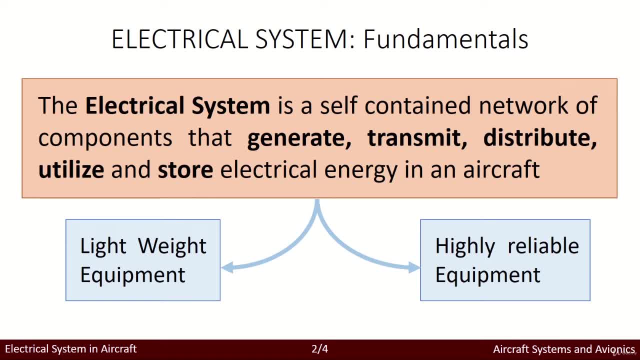 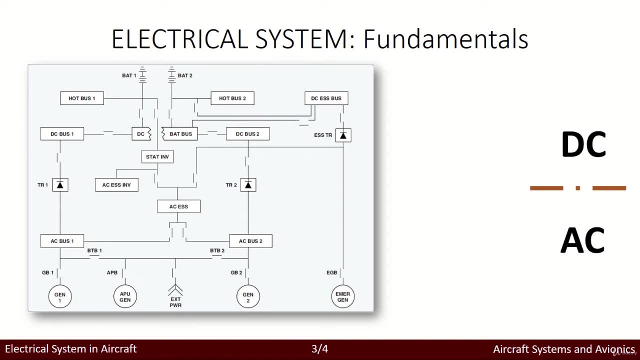 It is essential to make sure that all systems are lightweight and highly reliable. Okay, now, an airplane contains two major electrical circuits, which are usually named simply number one and number two. okay, and also an alternate circuit which may depend on, depending on the aircraft, or may depend on the type of aircraft, for instance. 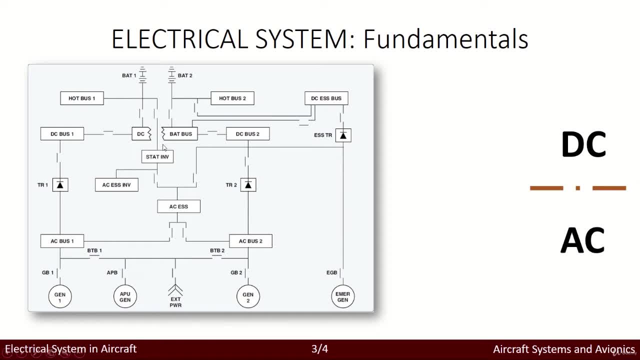 Now the two circuits, one of each side of the aircraft, are linked to a generator. It is this generator that will produce the electricity using the mechanical energy supplied by one of the engines. Okay, so each of the generators, generator number one and two, are related and are based. 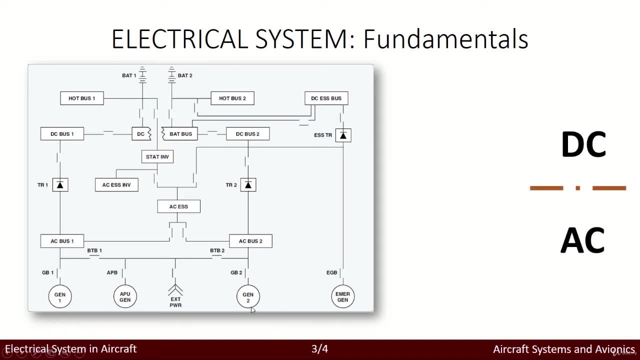 on the mechanical energy that we obtain from the turbines, from the aircraft engines. right, The electrical circuits used are based on different components. First of all, we have generators, as we mentioned before. Then we have the alternating current bus- okay, buses- which is the transmission of the current. 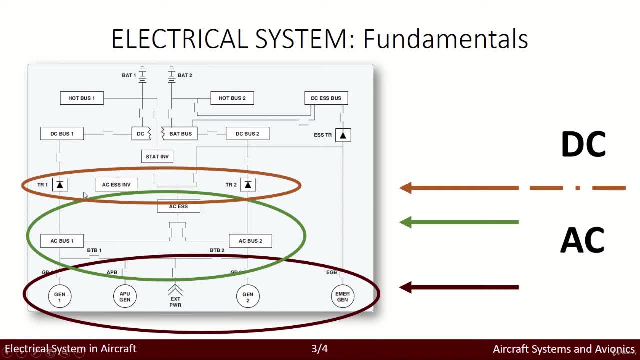 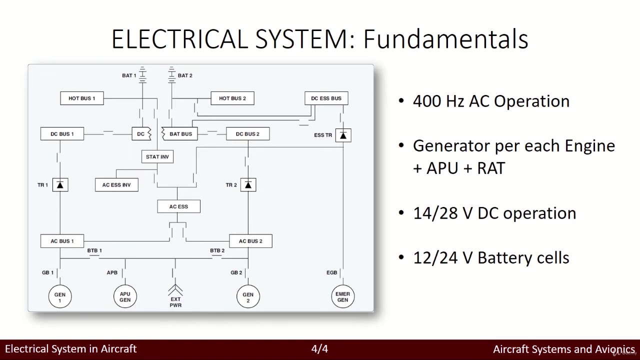 through alternating current. Then we have this area which is based on transformers, which we will explain in a bit, And finally this area over here, which is the most utilized in aircraft, which is based on DC current. okay, Right, so, as previously mentioned, electrical parameters are chosen to minimize the weight so the aircraft can get off the ground.